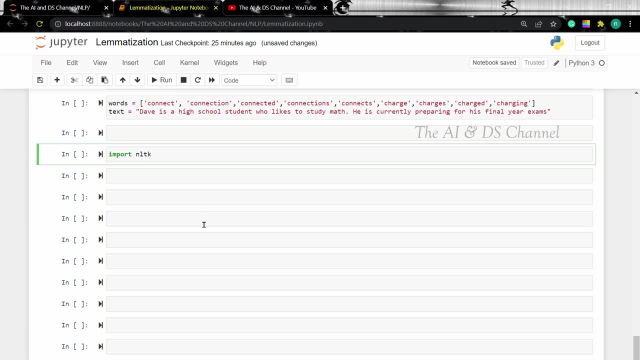 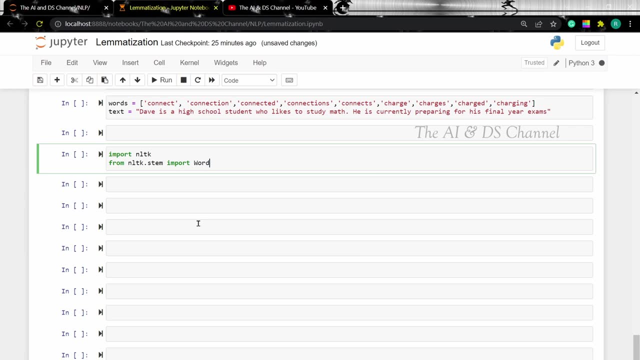 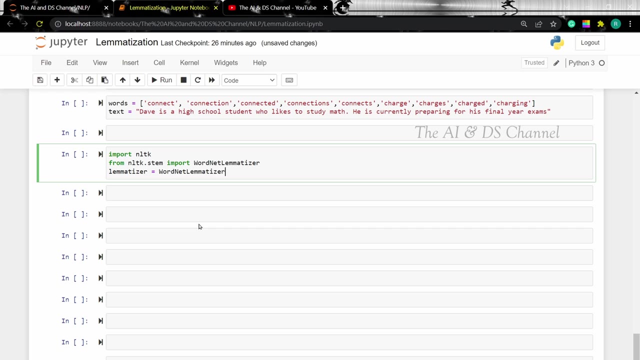 Now I have created a sample set of words and a sentence to perform lemmatization on. I'm using the same example that we use for stemming so that we can compare the results. Now let's perform lemmatization on the words. 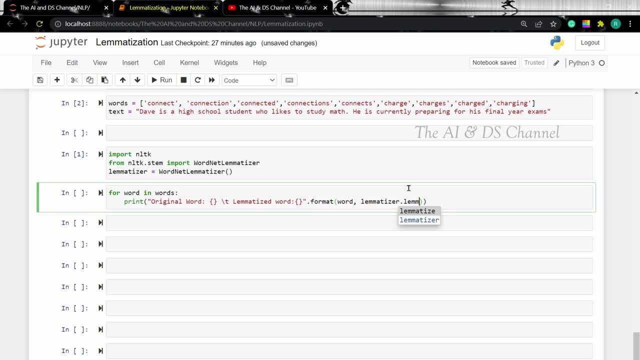 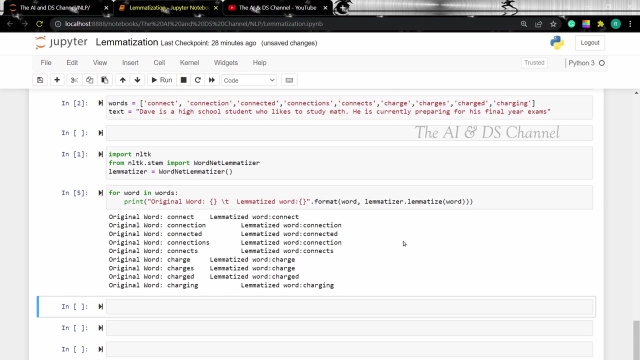 So what we are doing here is we are creating a volume that goes through each word in our words list and then prints the original word along with the lemmatized word. And now let's run it. As you can see, all the words are reduced to their root forms. Now to show you how it differs from: 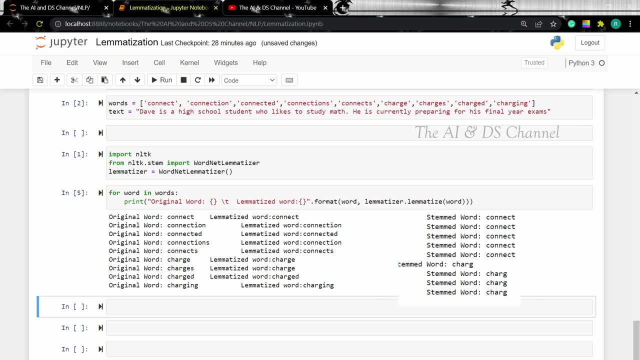 stemming. I will show you how to do that. So let's go ahead and import the NLTK and load the NLTK. I'll add a screenshot of the output that we got when we performed stemming on the same words. Now, if you want to check out my video on stemming, I'll add a link to it in the description below, as: 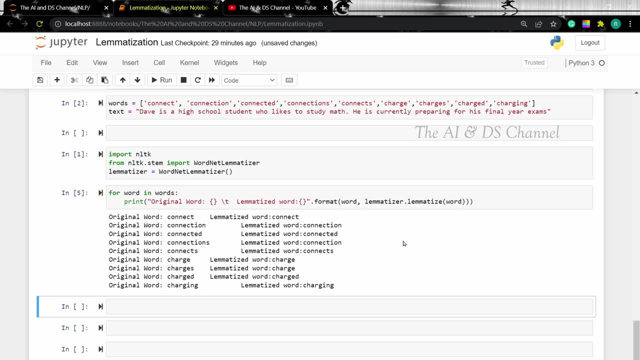 well, Let's now perform lemmatization on the sentence. So, as I said in the previous video, the input to the lemmatizer must be a tokenized text. So to do that, first we need to tokenize the text data. 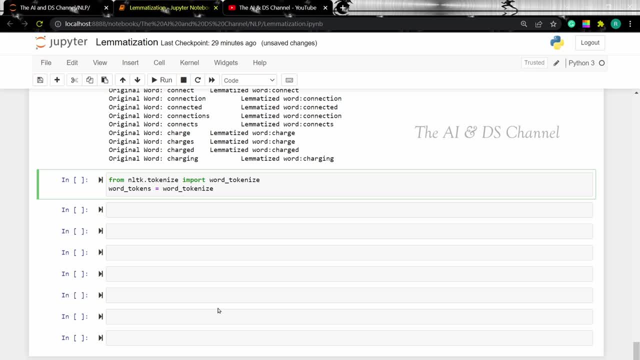 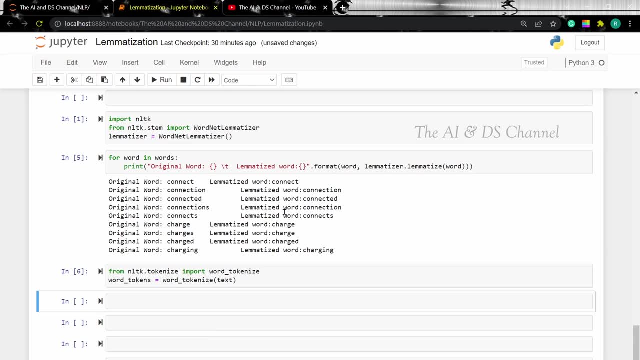 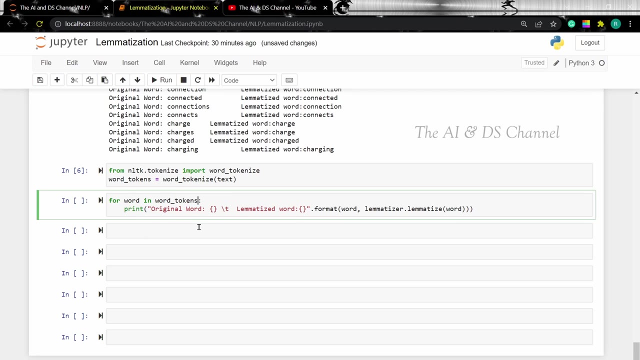 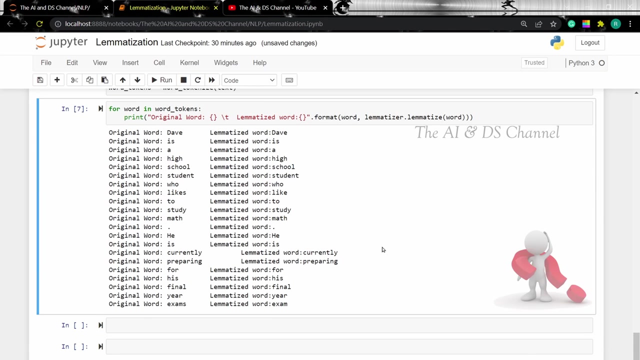 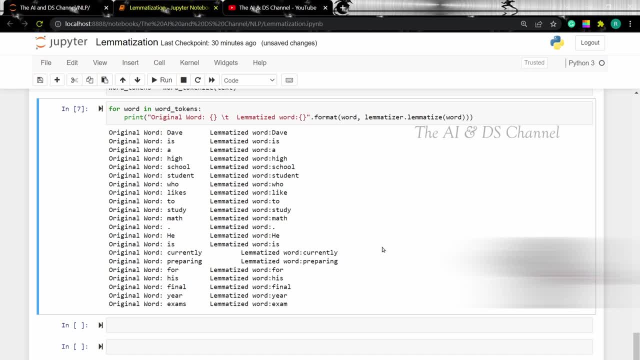 look. Can you spot the difference? Let me know. in the comment section below I'll also add a screenshot of the output that we got when we performed stemming, so you can have a better understanding of the two techniques. Now, when you perform lemmatization, the output changes when you specify the context. This is done by